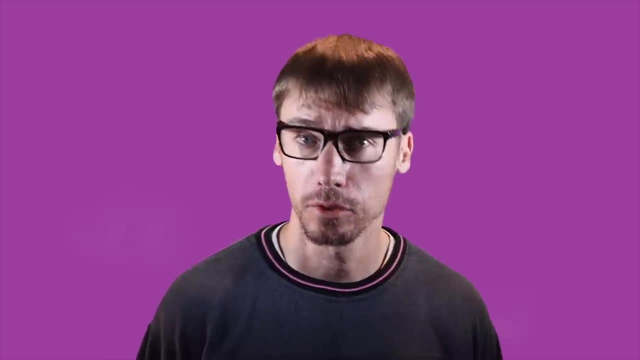 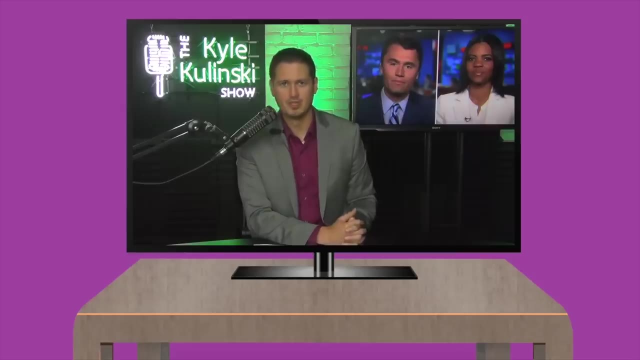 I'm Mr Beat. Let's watch some people talk about politics, shall we? Charlie Kirk and Candace Owens, the right-wing superstars, went on Fox News and what they did is they spewed the most boring, banal right-wing talking points I've ever heard. 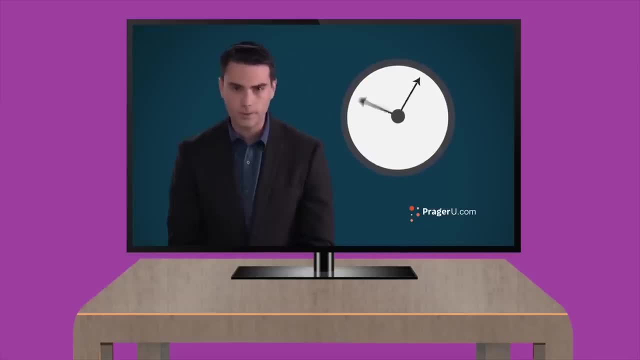 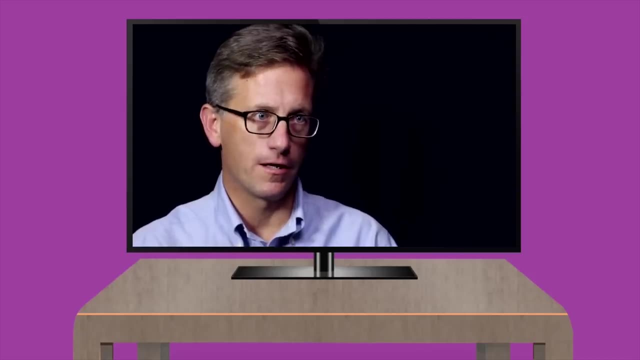 They spin out hour after hour of slickly produced left-wing propaganda And those people have more or less systematically been ignored by people on both the right-hand side and the left-hand side of the political spectrum. On the right- conservatives- you're always talking about taxes and regulations and big 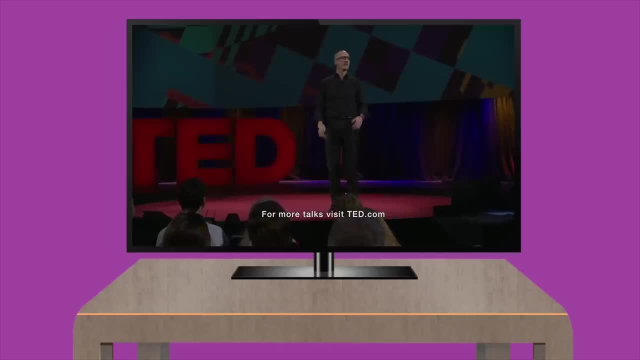 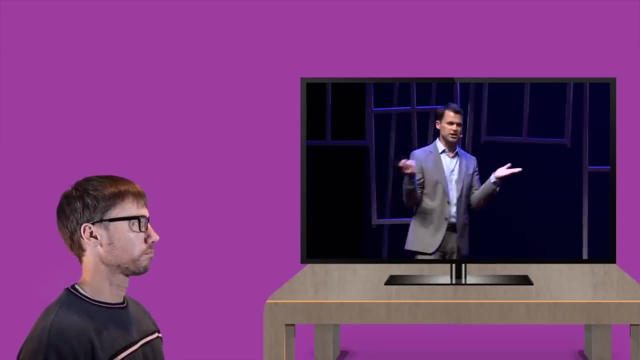 government And, on the left, liberals. you're talking about economics. It's always about income inequality. right, The divide between the left and the right is as bad as it's been in really any of our lifetimes. You know what? I'm not quite sure that all of these people have the same definitions of 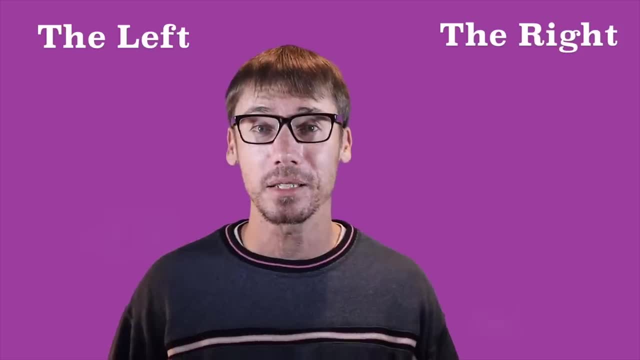 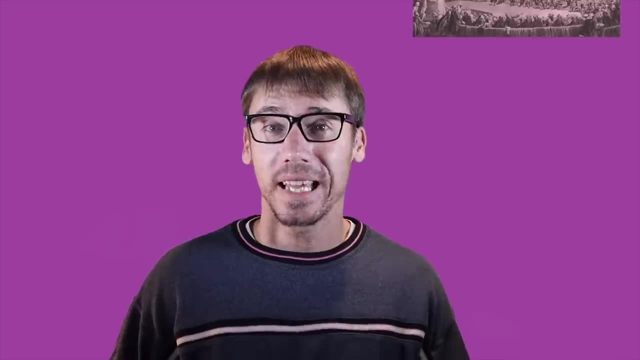 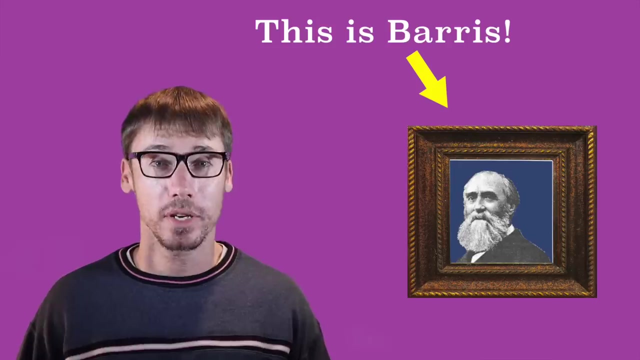 the left and the right. What do people mean when they say left-wing or right-wing? Well, the whole political spectrum that gave us left versus right began during the French Revolution not that long ago. For more about this, I'm going to send you to Mr Barris from the channel. This Is Barris. 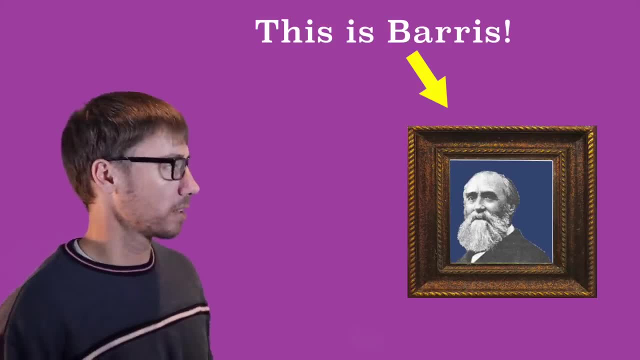 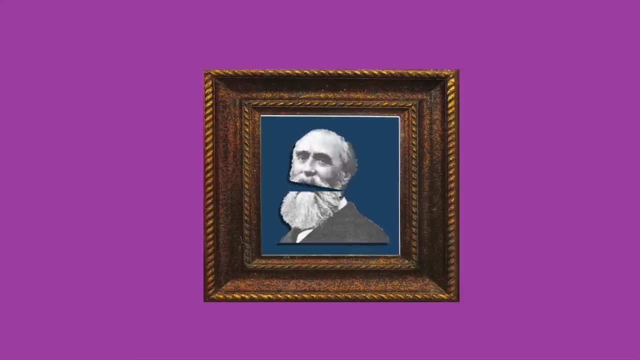 He's going to get into the history of why we have these terms. Go ahead, Barris. yeah, Thank you for having me over Mr Beat. To discover the origins of the left versus right paradigm, one must go as far as the French Revolution, with the creation of the National 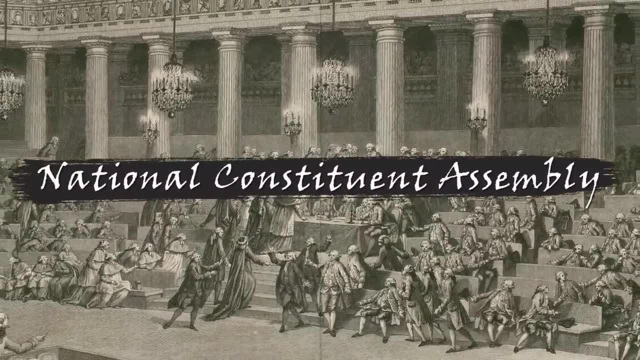 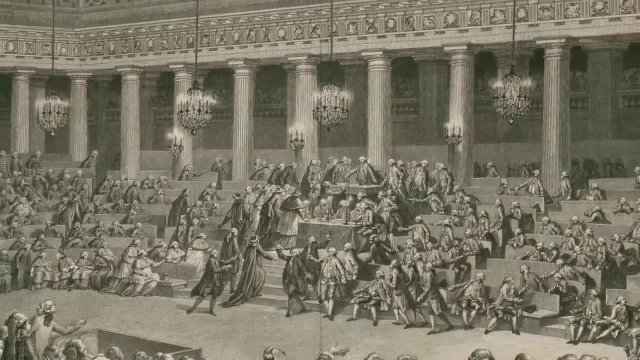 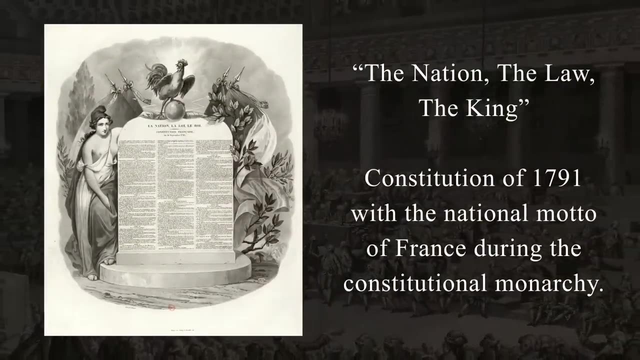 Constituent Assembly whose main task was to draft a constitution. Now, while France is proudly republican today and any trace of royalty has long been guillotined away, that wasn't always the case, and a large portion of the population supported the king, or at least those who represented that population. 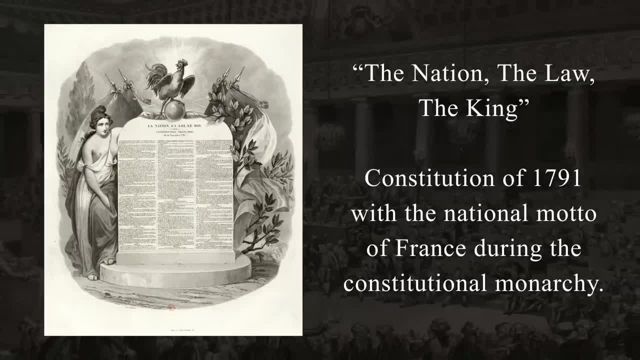 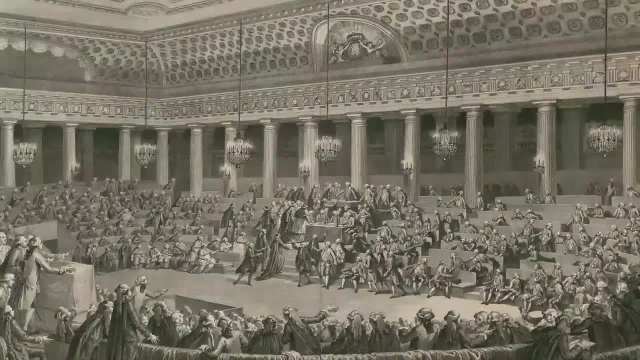 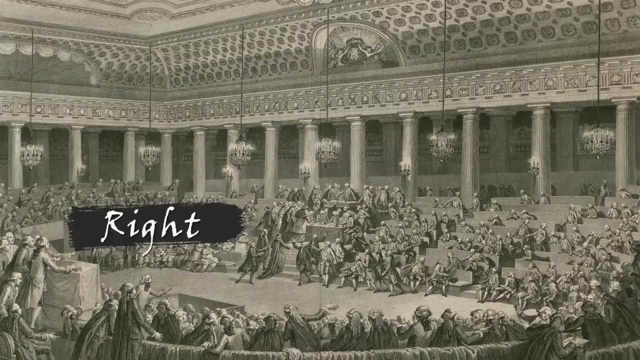 As such. when, on November 11, 1789, the Assembly had to vote on whether the Constitution would grant the king an absolute veto or a partial veto, those who favored an absolute veto were asked to sit on the right of the president of the assembly, while those who favored a partial veto, which was 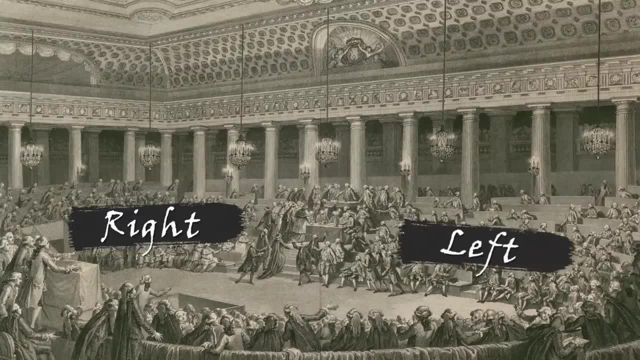 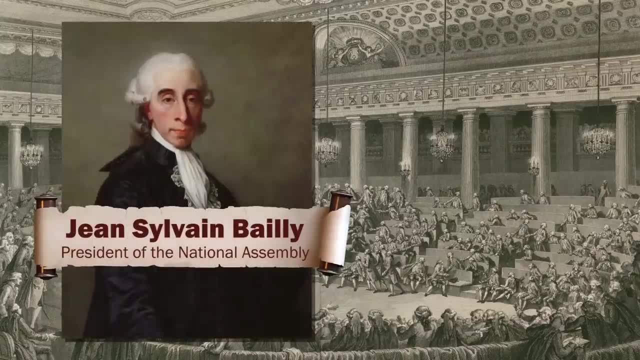 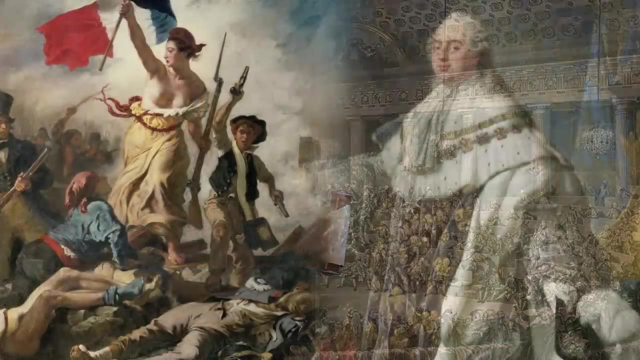 the more radical position were asked to sit on the left. This wasn't done symbolically but to make the vote count easier for the president, who felt a bit overwhelmed by the 1500 deputies. And just like that, France started this idea of change versus tradition of liberalism. 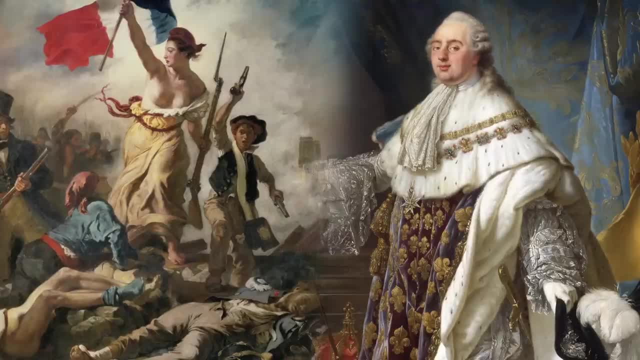 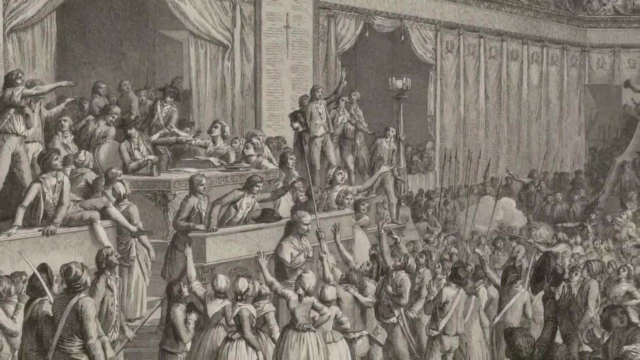 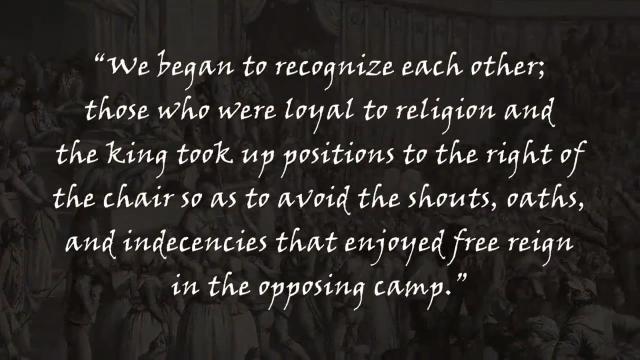 versus conservatism, which still shapes the political landscape to this day. In the following months, the deputies will maintain that distinction, not out of ideology but rather necessity. as the baron de Gauville explained, We begin to recognize each other, those who were loyal to religion and 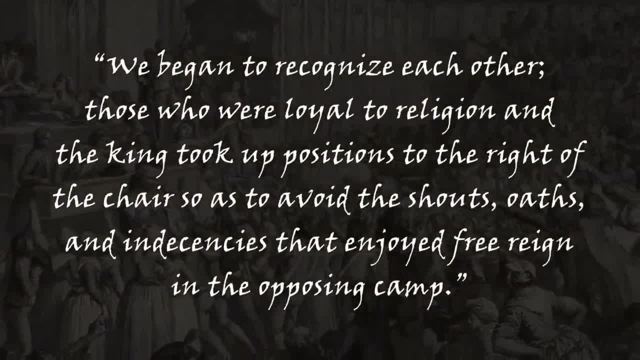 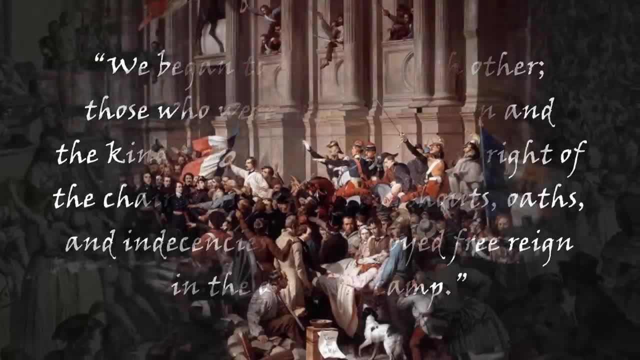 the king took up positions to the right of the chair so as to avoid the shouts, oaths and indecencies that enjoyed free reign in the opposing camp. Furthermore, being on the same side of the political system, France will continue to be a political leader and it will continue to be a political leader. 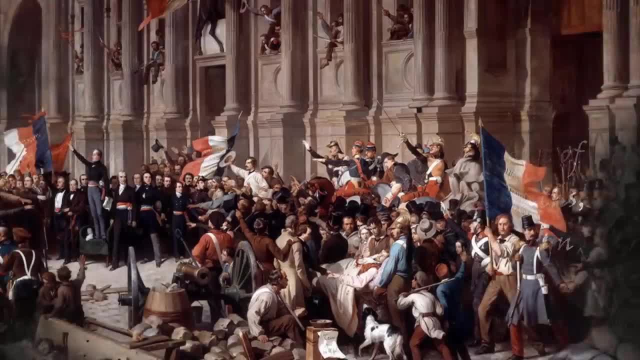 The French will continue to be a political leader and it will continue to be a political leader. The French will continue to be a political leader and it will continue to be a political leader. spectrum by no means meant that you shared the same ideologies. It is often forgotten that the 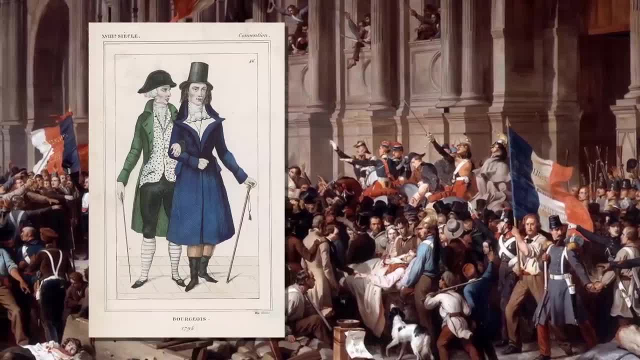 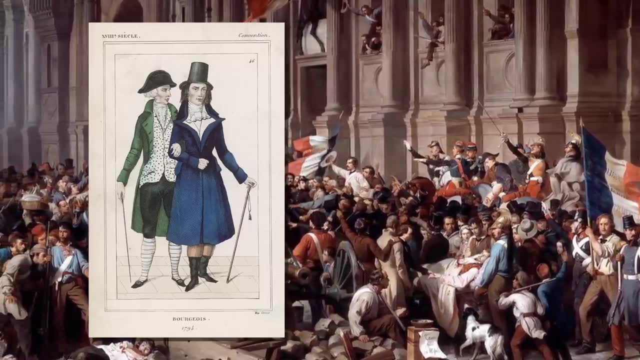 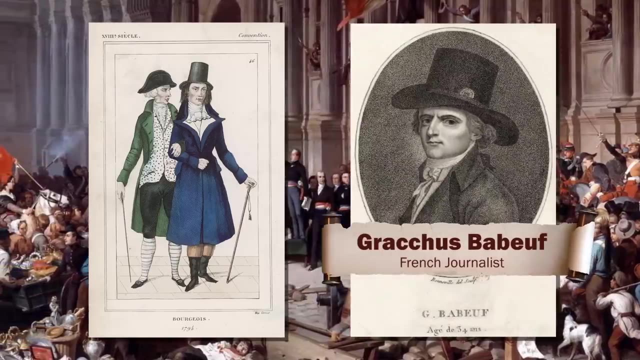 French Revolution started as a bourgeois revolution. The bourgeois were somewhat republican and thus considered left-wing. However, most bourgeois also supported free market reforms and liberalism in the classical sense. And when you have proto-communists like Cassius Babuff, who were also considered left-wing because, well, the alternative meant support of the king. 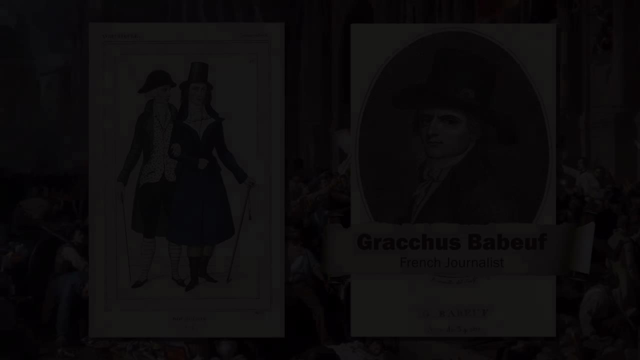 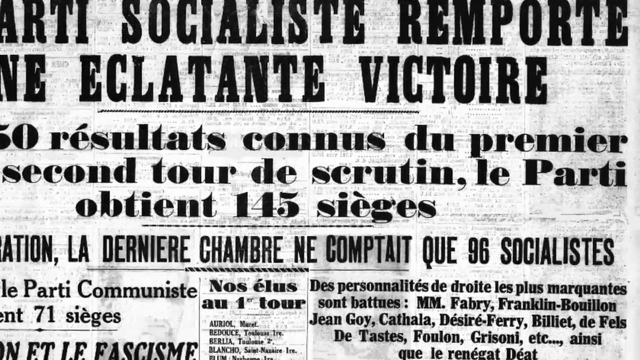 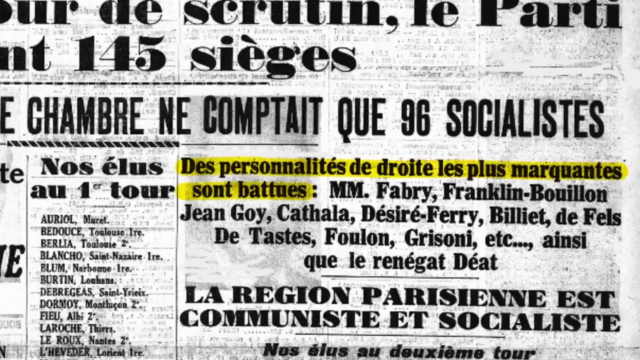 you get why this might be problematic. right, It would take another century before the left versus right spectrum became popular outside of France. In the beginning of the 20th century, as revolution sprouted across the world, the press and academics needed a quick way to categorize the 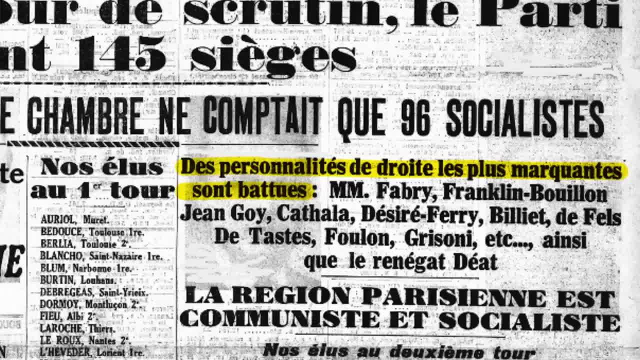 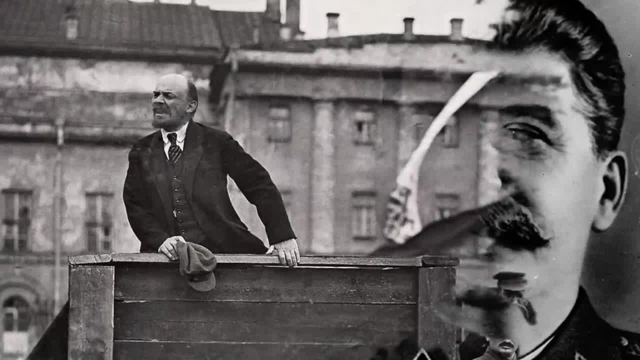 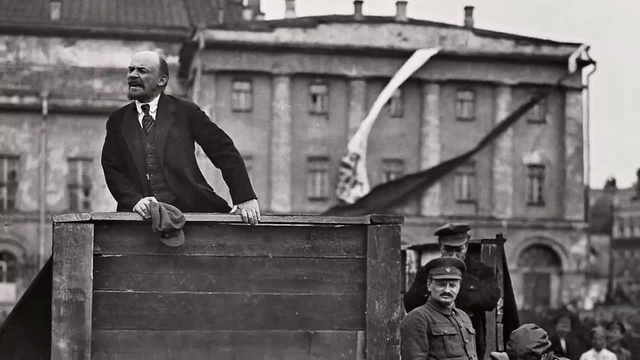 different ideologies that were fighting each other, especially as these ideologies, both left and right, became increasingly radical. For example, the Bolsheviks, who loved anything related to the French Revolution, were more likely to support the French Revolution, immediately embraced the left-wing versus right-wing spectrum, although they considered 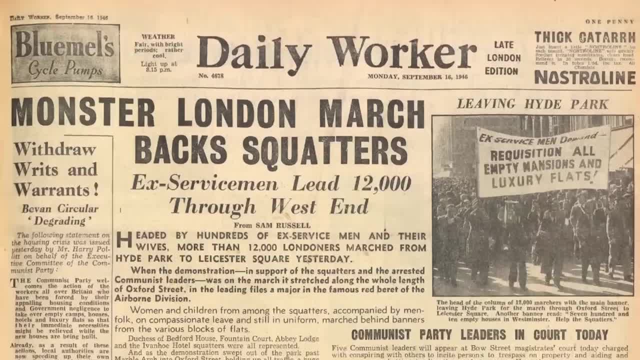 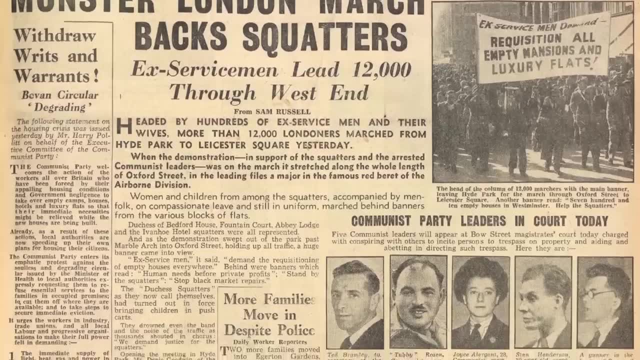 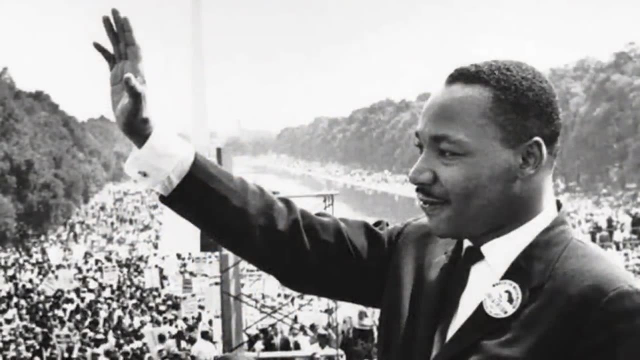 themselves the centrist position. In England, however, the political spectrum took longer to become widespread and books only started referencing it in the late 1920s. Adoption in the US was just as slow, but eventually, as partisanship increased in the 1960s, during the 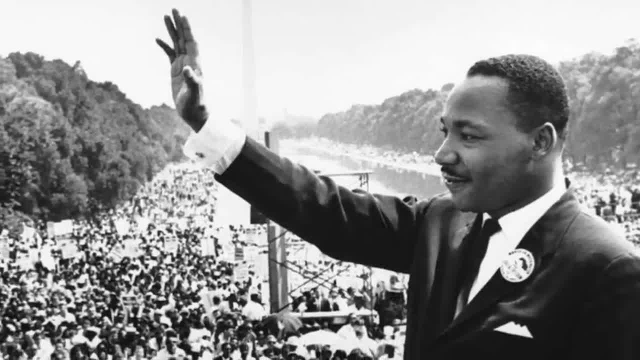 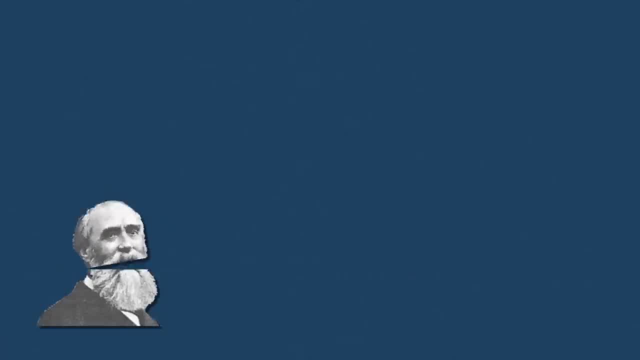 civil rights movement. the idea of a left versus right political spectrum cemented the idea of a left versus right political spectrum cemented along the beliefs of both parties. And that's it, Mr Beat. That's the story of how an overwhelmed president who needed an easier way 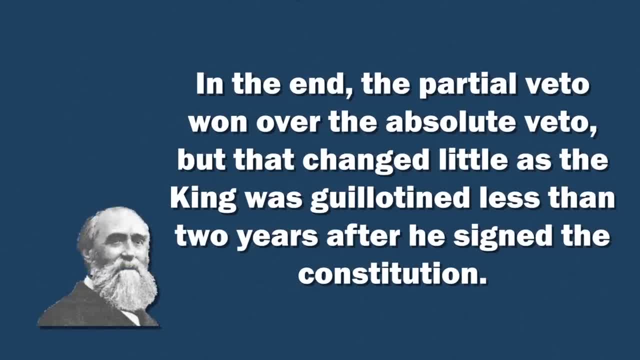 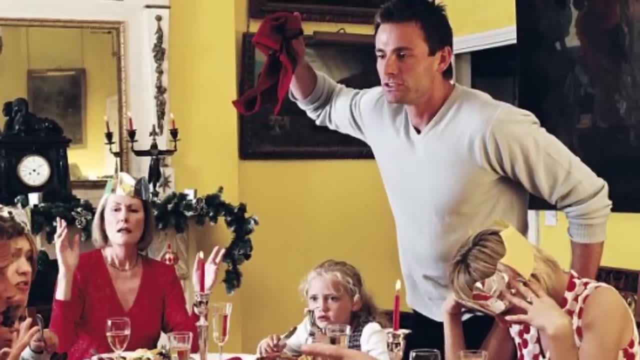 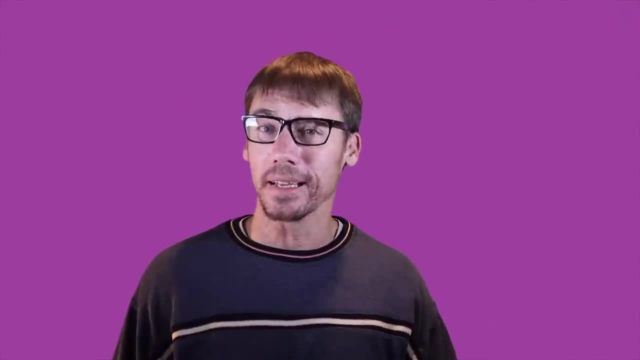 to count. his deputies ended up creating a system which now allows millennials to dismiss their uncle as a racist right-wing boomer, while he dismisses them for being triggered left-wing snowflakes. Well, thank you, Mr Barris. What about today? eh? 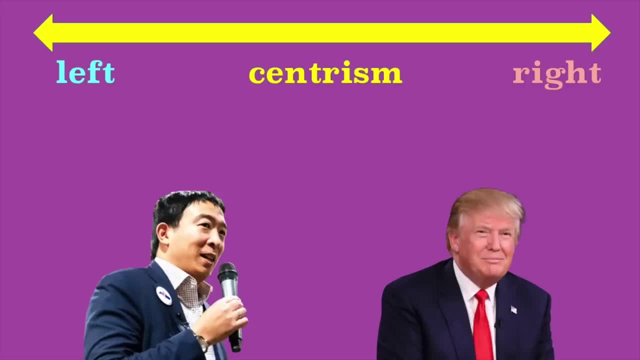 Well, often the political spectrum looks something like this: On the left side of politics, you tend to see ideas like Liberty, Equality, Progress and Internationalism. On the right side of politics, you tend to see ideas like Authority, Hierarchy, Tradition and. 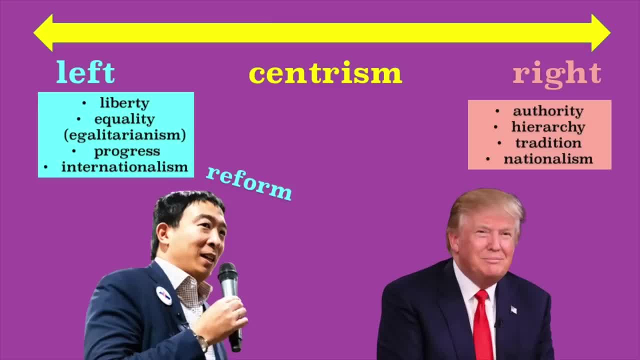 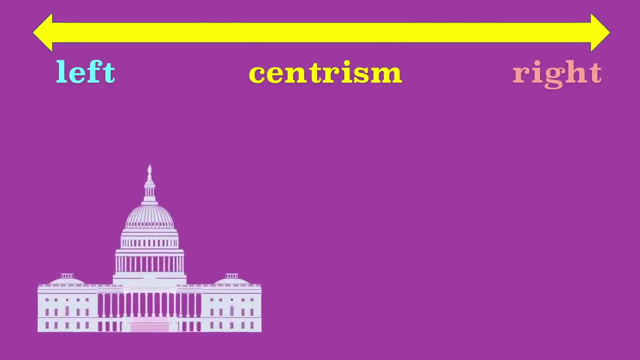 Nationalism. On the left, you often see Reform, while on the right, you often see Reaction. Those on the left tend to want more government involvement to make society better- They want an more top-down- while those on the right tend to want less government involvement to make 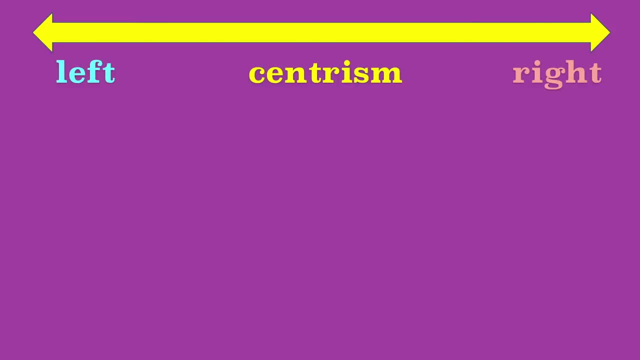 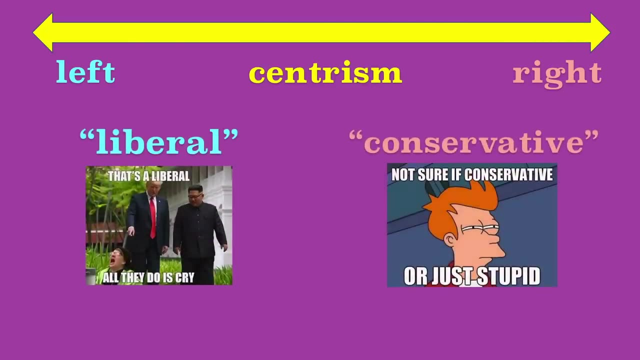 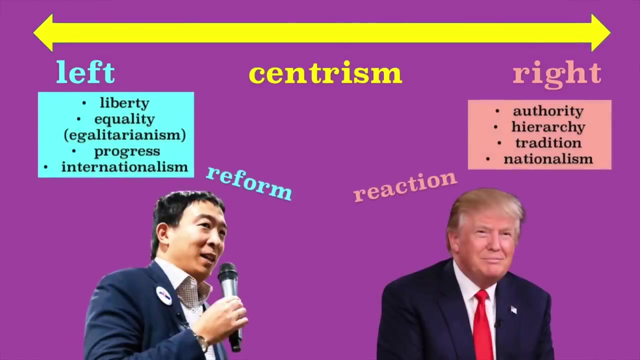 society better They want it. bottom-up Ideas on the left are often called quote liberal and ideas on the right are often called quote conservative. Of course, these generalizations are incredibly misleading, which is why this political spectrum is pretty much crap. 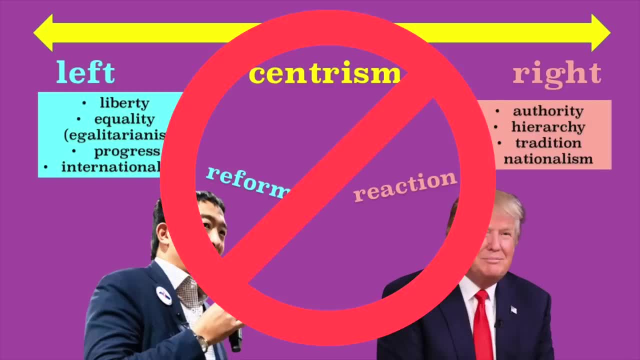 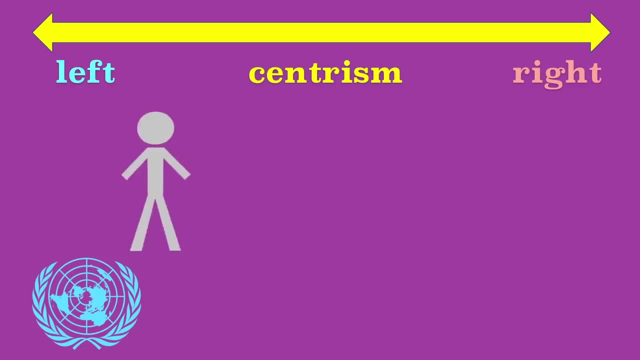 I mean rarely do folks fit neatly on one side or the other. For example, a person might think the government generally screws everything up when it gets too involved, yet absolutely hates nationalism or hierarchy. Often folks find themselves caught up with this weird label called quote centrism. 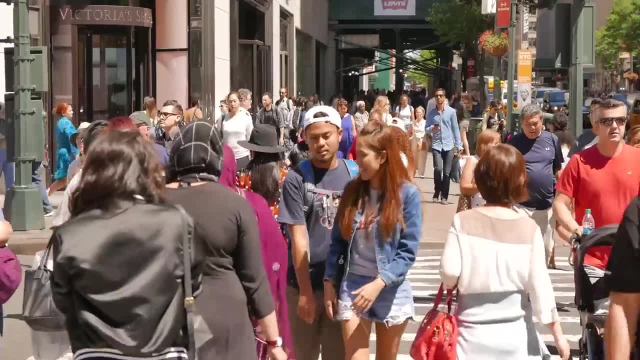 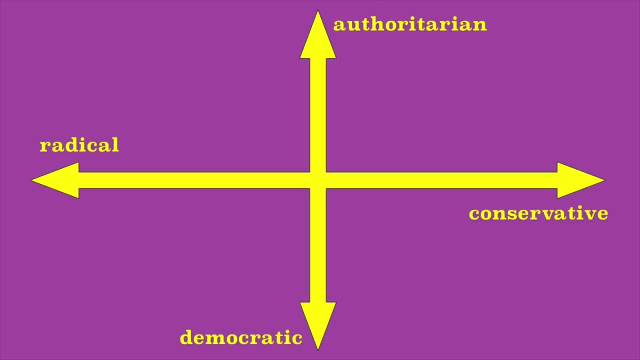 because they fall somewhere in between. However, most people fall quote in between on most issues. Hey, can we get a better political spectrum up in here, please? Thanks, Ok, what's this one? Oh yes, This one was developed in the 1930s. 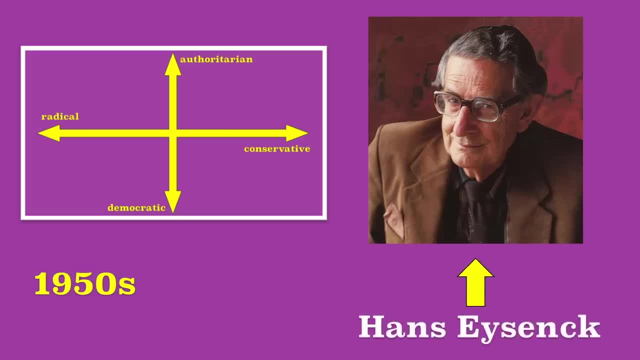 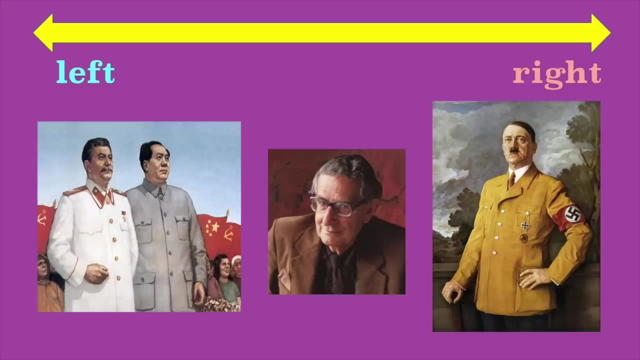 It was developed in the 1950s by a psychologist named Hans Einsink. He noticed that there was something similar going on with the Nazis, who were supposed to be on the right end of the spectrum, and communist dictators who were supposed to 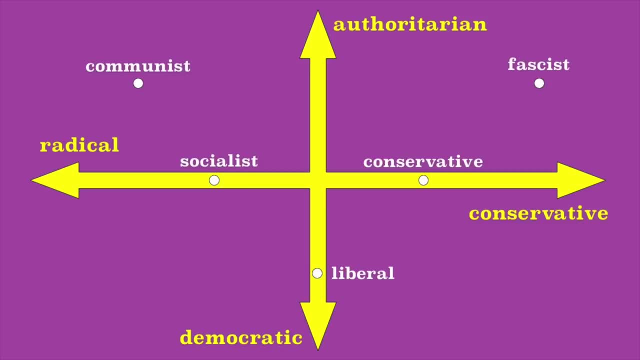 be on the left end of the spectrum. So he came up with these two spectrums: an R factor representing radicalism, and a T factor representing tender-mindedness. Needless to say, Einsink's diagram had its critics, In particular this dude. 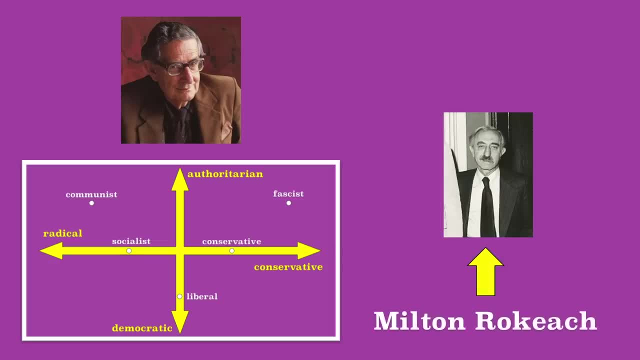 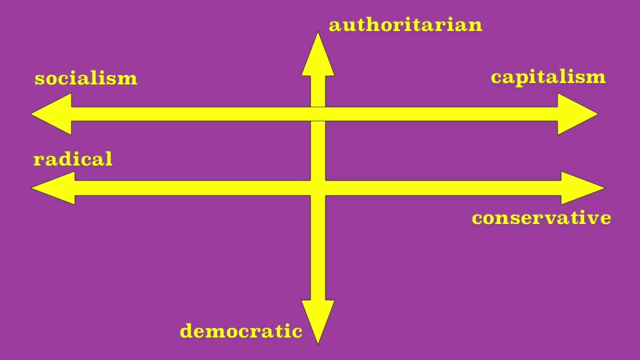 Another psychologist named Milton Rokic, who argued the big difference between the left and right was basically that the left stressed equality more. Needless to say, Einsink later adapted his chart to look like this, bringing an S factor spectrum which followed economic beliefs. 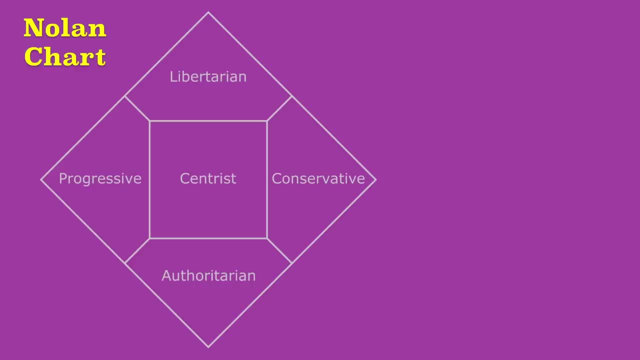 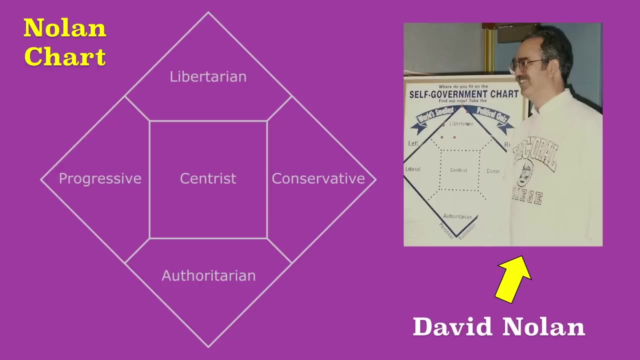 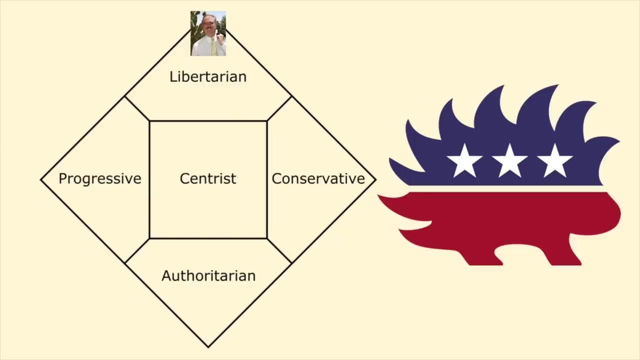 Around. that same time, the Nolan Chart, developed by a libertarian activist named David Nolan, became a handy way for people to quickly see where they fell politically by looking at a personal freedom spectrum and an economic freedom spectrum. Yep, that's about where Nolan would have been on his own chart. 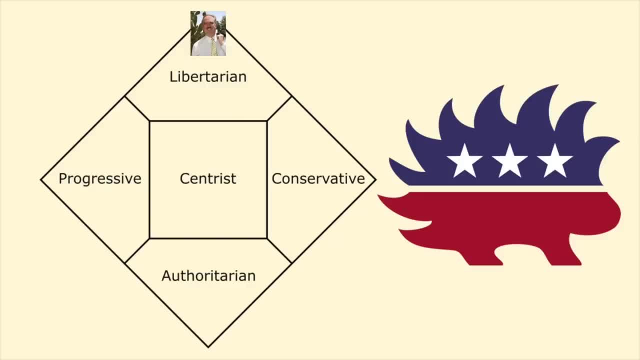 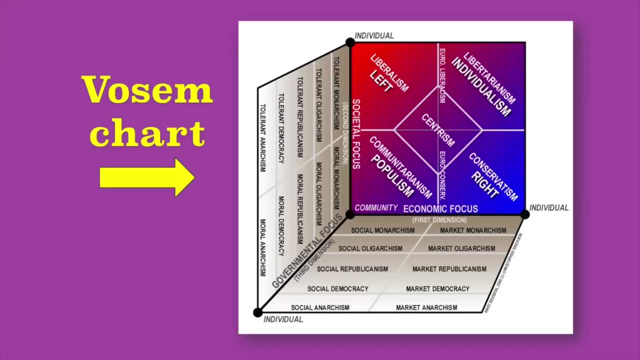 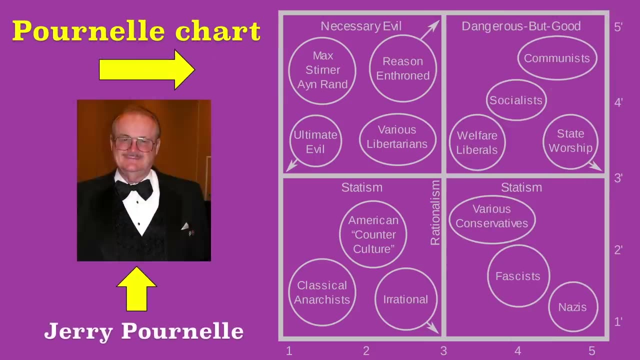 And, yes, today it's still heavily used in libertarian circles. The Vosum Chart was a three-axis version of the Nolan Chart and looks like this: Whoa, that one looks complicated. Other two-axis charts include the Pornel Chart, developed by this dude, Jerry Pornel. 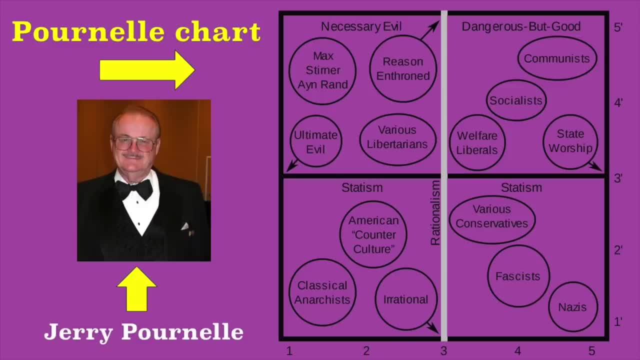 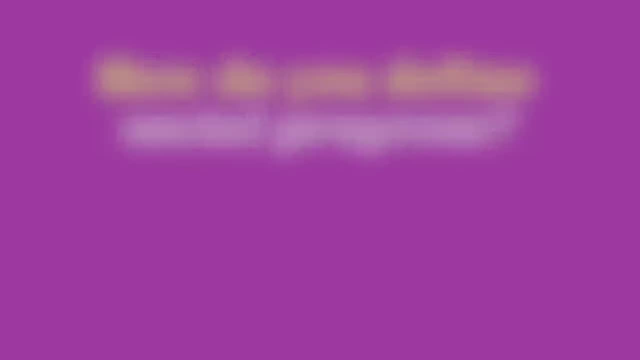 The Pornel Chart or, as he said, the state On the other people's attitudes toward social progress. But wait a second. How do you define social progress, though? Over the years, there have been tons of political spectrum charts like this one and this one. 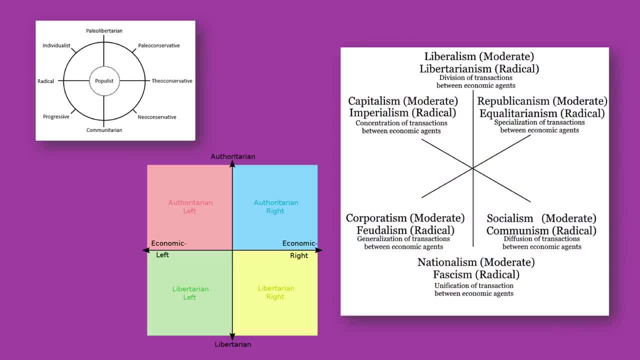 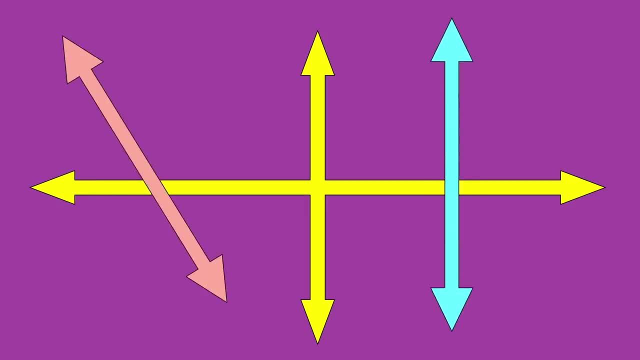 and more three-axis versions like this one. But the problem is, people won't stop fighting about which chart is best. Most of the debate centers over which axis or axes to include for each one. Wait a second. The plural of axis is axes. 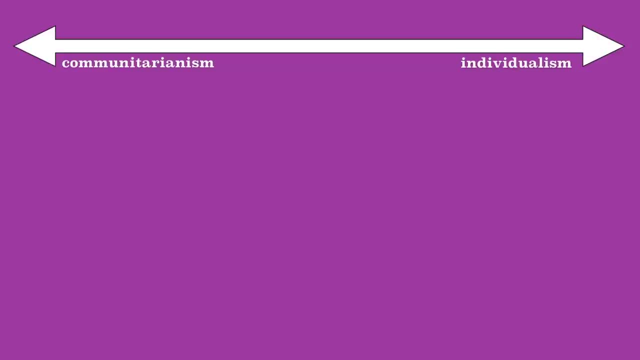 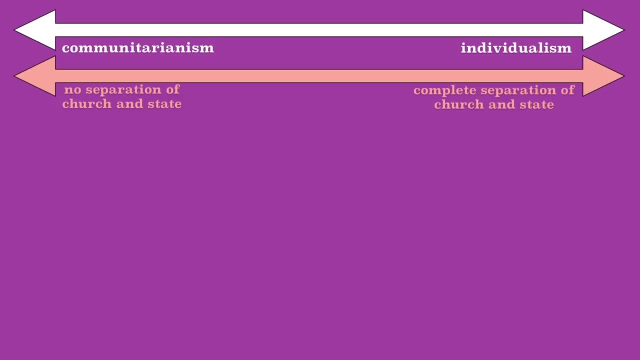 What the heck? Anyway, additional axes include Communitarianism vs Individualism, No Separation of Church and State vs Complete Separation of Church and State. Interventionist Foreign Policy vs Non-Interventionist Foreign Policy. Multilateralism vs Unilateralism. 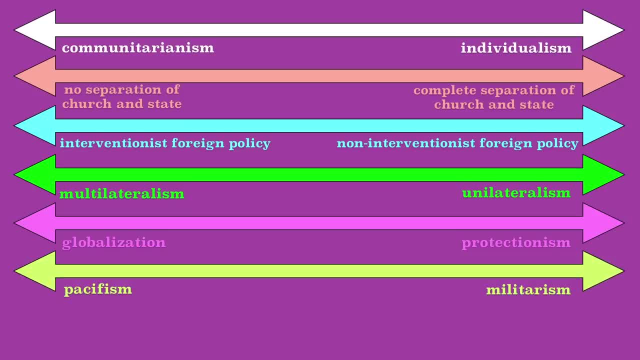 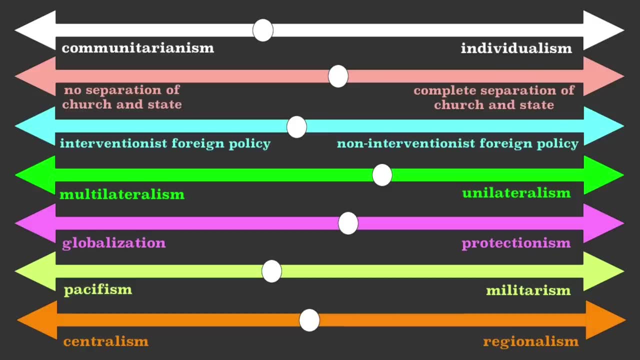 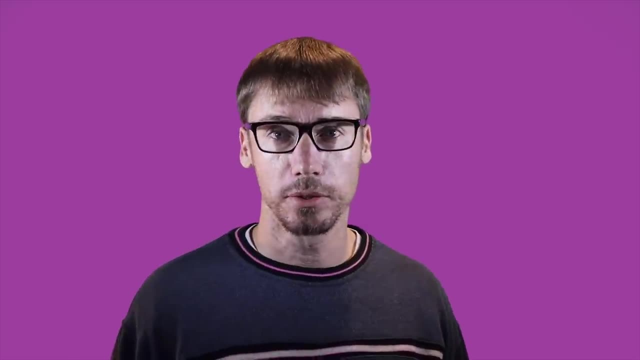 Globalization vs Protectionism, Passivism vs Militarism and Centralism vs Regionalism. That's a lot of isms. Again, odds are: almost all of you are somewhere in the middle on all of these spectrums. So where do you fall? on the political spectrum, 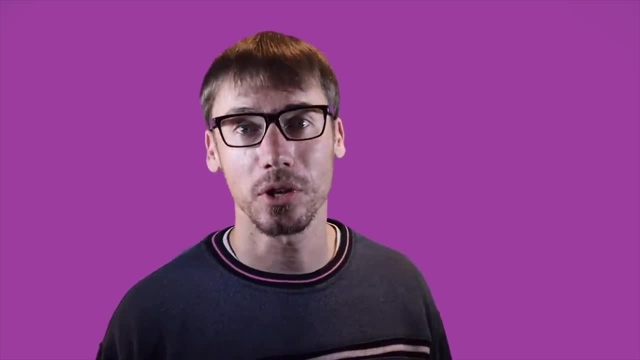 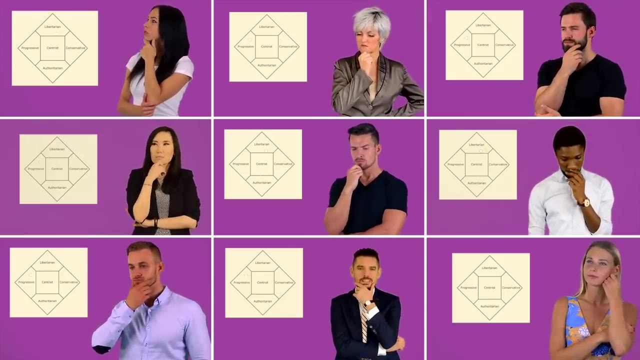 That's right, you With the yellow shirt. Well, I think it depends on the issue. It's not static. Chances are, you are constantly moving around on the spectrum And that's probably a good thing, because it shows that you have a more open mind.